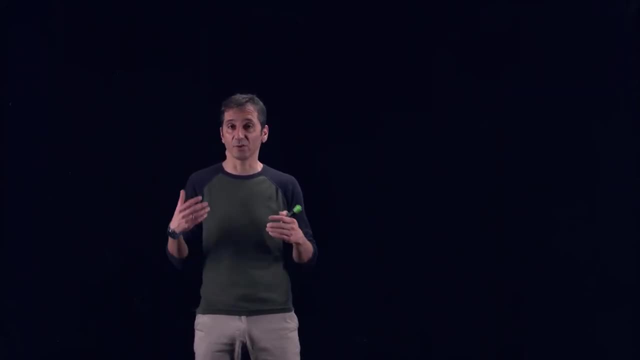 including to cooling down and keep fresh, actually, your food, medicines and drinks also, since the videos that you are watching are recorded in 2021, so during the pandemic. so COVID-19 pandemic refrigeration cycles have dragged a lot of attention, and why? because of the vaccines, and more specifically the Pfizer BioNTech vaccine. 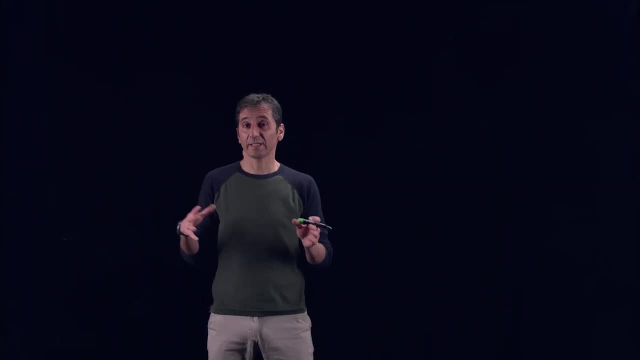 and the Moderna vaccine. they have to be kept at a very low temperature of minus 80 degrees C. so you can imagine the complexity of logistics. so, and our role actually in this chapter is to understand refrigeration cycles. okay, so we'll start with a simple refrigeration cycle and then we'll make it more. 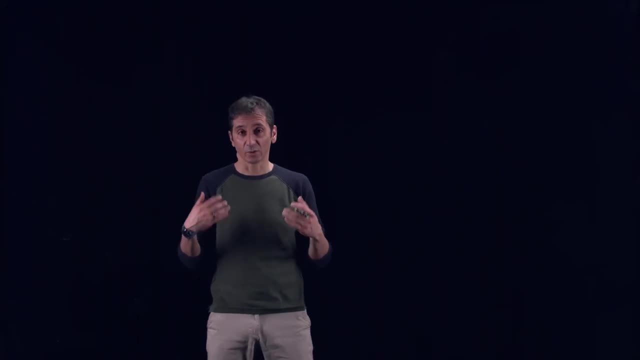 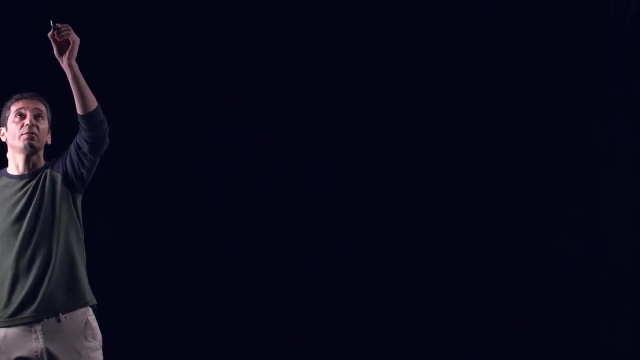 complex. okay, let's say, if we would like to go further down in terms of temperature, what do we have to do? and also, if we have to want to scale up our refrigeration cycle, what do we have to do? so what we'll be discussing in this chapter are refrigeration cycles. 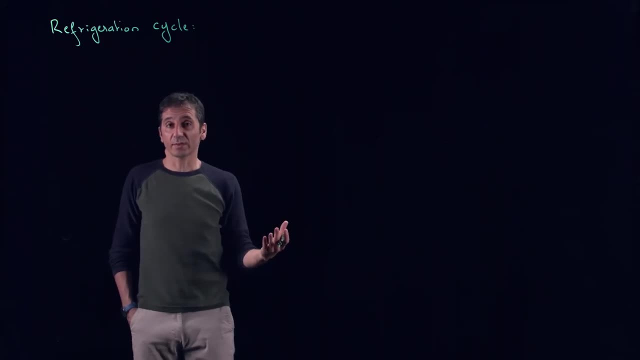 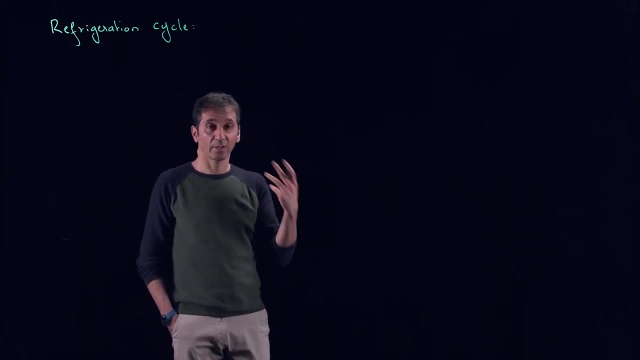 interestingly enough, we don't start actually from nothing because we already have a knowledge regarding refrigeration cycles, because in thermodynamics one, when we try to introduce closest statement of the second law of thermodynamics, we defined a carnal refrigerator and this is what we'll be. 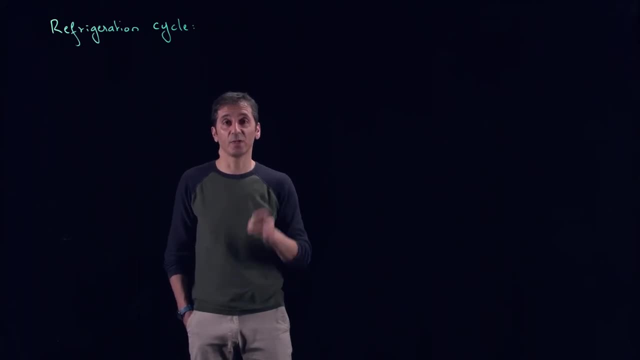 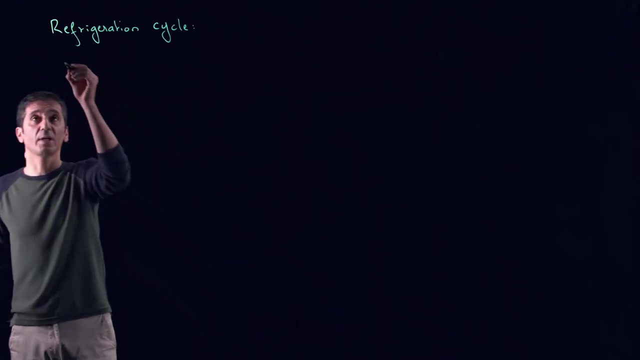 doing now. we'll be going back to our carnal refrigerator then to understand different processes and then we will understand why it doesn't work or why we cannot make work, and this will lead us to a more realistic refrigeration cycle: vapor compression cycle. so, if you remember well, our carnal refrigerator, 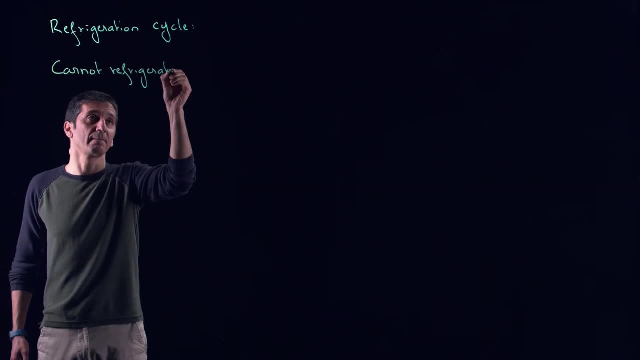 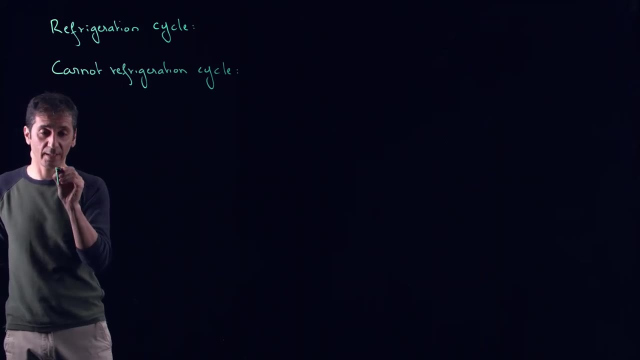 carnal refrigeration cycle. the schematic diagram was that. what do we have? we have a low temperature reservoir and a high temperature reservoir. so this will represent the designated gas and the requested form of the equationnovation phase. This specialization equation is called inspect. As you hear that part of that is called inspect. 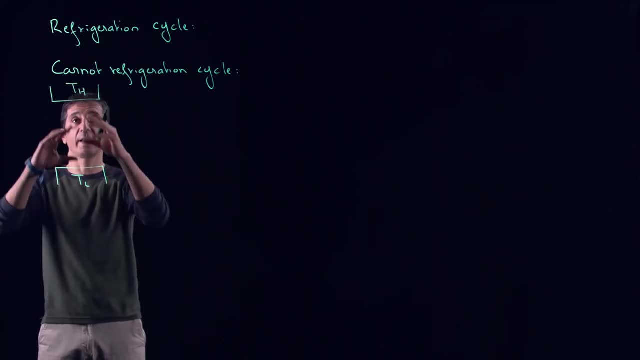 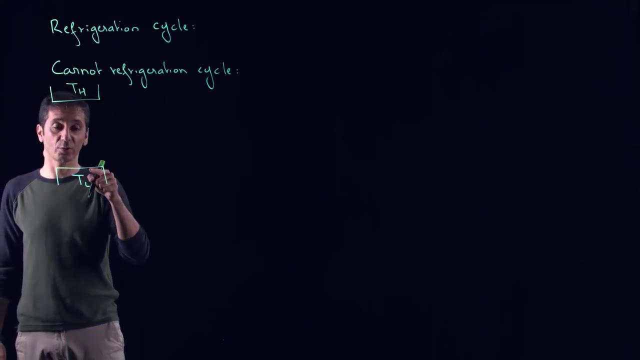 for example, inside the cabinet of your fridge, and th will represent the surroundings, okay, the kitchen, a room, apartment or whatever. and our role in refrigeration cycle is to get heat out of the cold and send it to the hot. okay, and Clausius told us that the only way to do this. if you want to go against, 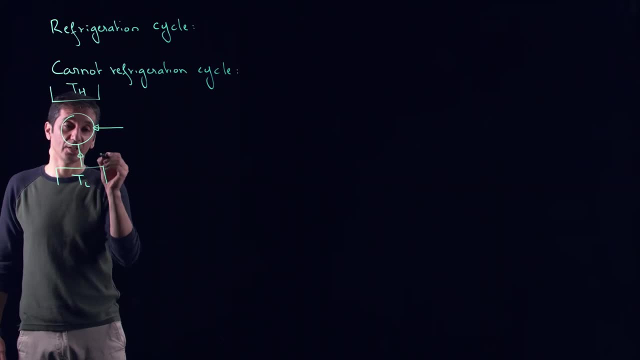 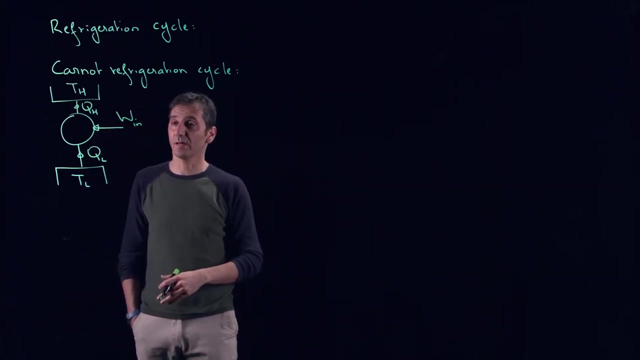 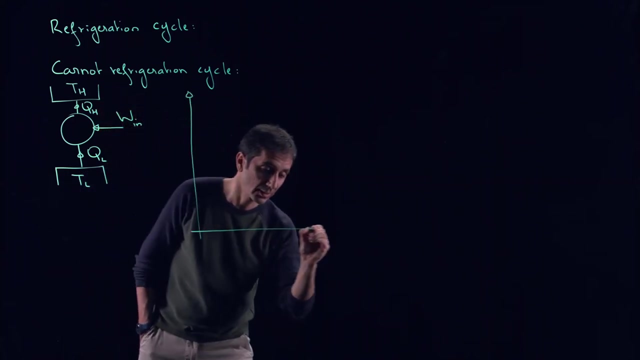 nature from cold to hot and therefore extract a QL and reject it into a Q H. there is a price to pay and the price to pay is work in, okay. so now, basically, if I have to sketch a TS diagram for our carnal refrigerator, we have a refrigerant, okay. 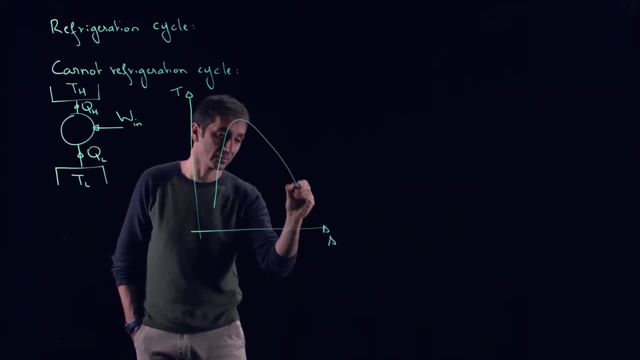 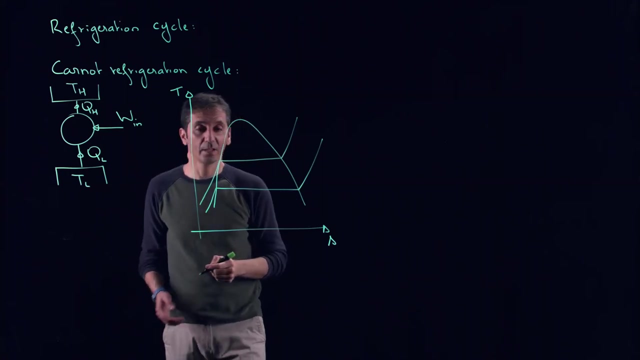 so therefore, now, basically, if I have to sketch a TS diagram for our carnal refrigerator, we have a refrigerant, okay so therefore we'll have to go back to our bell curve or the dome, and we are playing between two different pressure lines. okay so, and the schematic diagram will be that in a 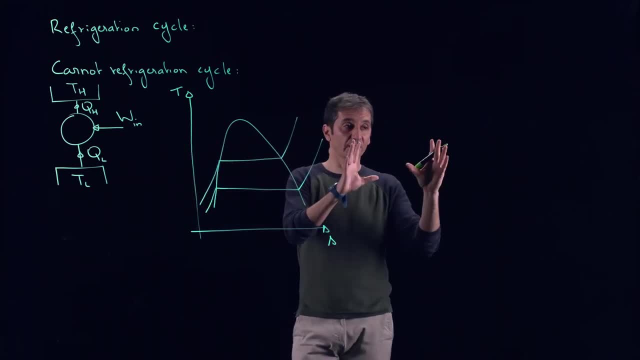 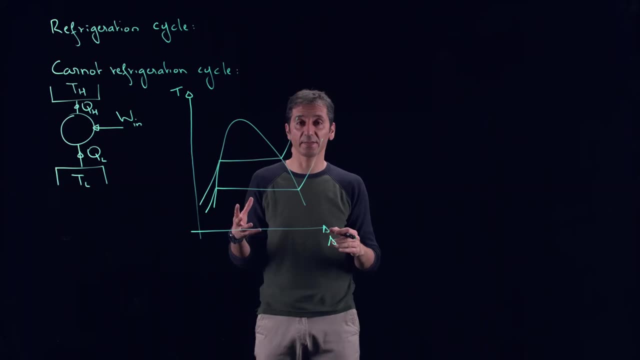 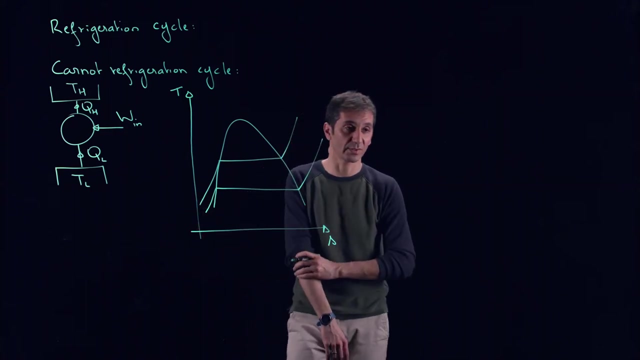 corner refrigerator. so we can still sketch something like a power cycle and reverse it. because Carnot is a reversible cycle, meaning that if you turn it in one direction you have a power cycle. you're rotating. in the other direction you have a refrigeration cycle. so then we can still use the same. 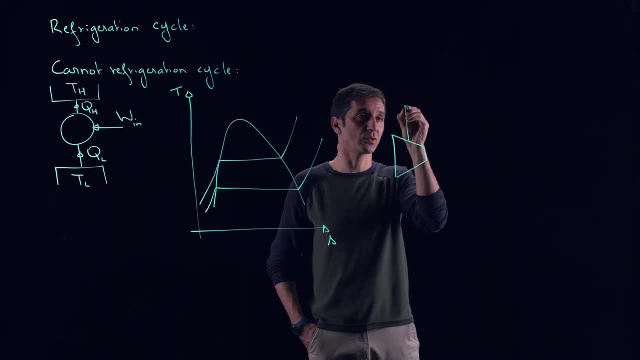 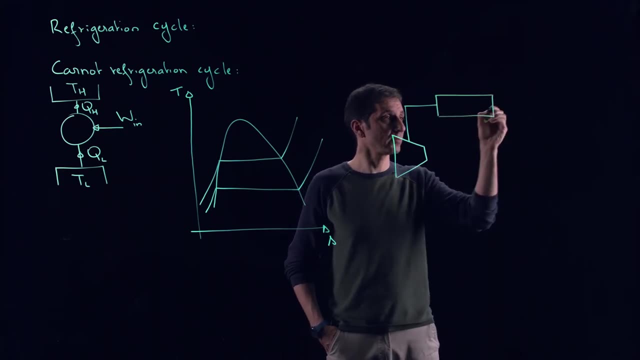 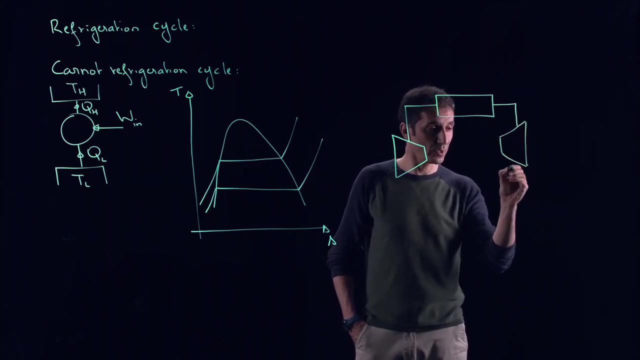 schematic diagram. as for our power cycles, okay, so we have here something let's say to to provide work. we have here kind of a heat exchanger- we will give the different names- and here we are providing work. this is for a power cycle and we are rejecting. 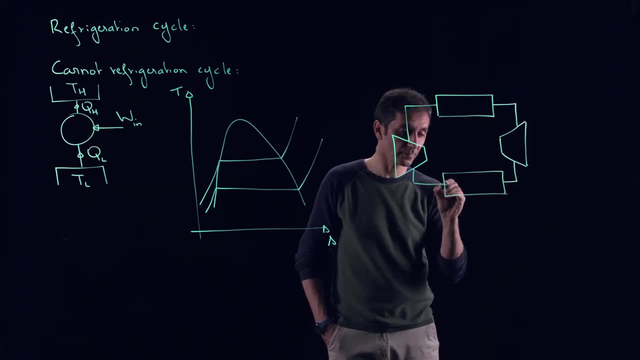 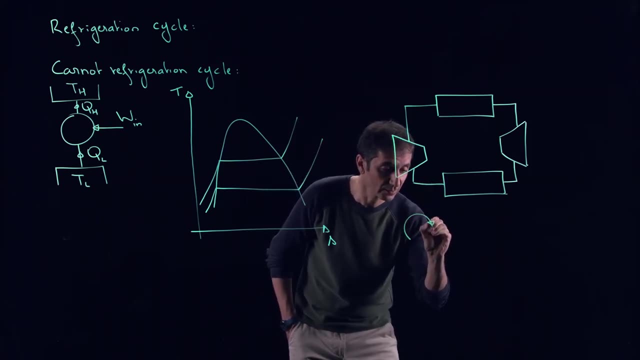 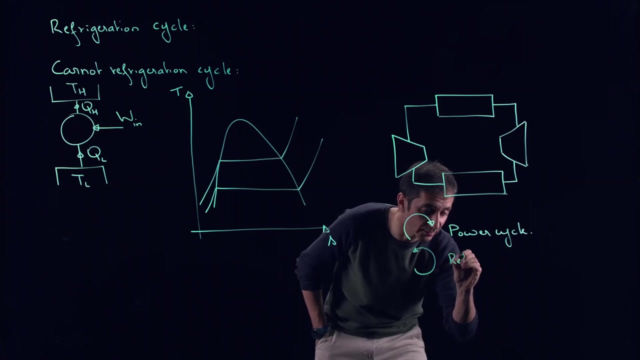 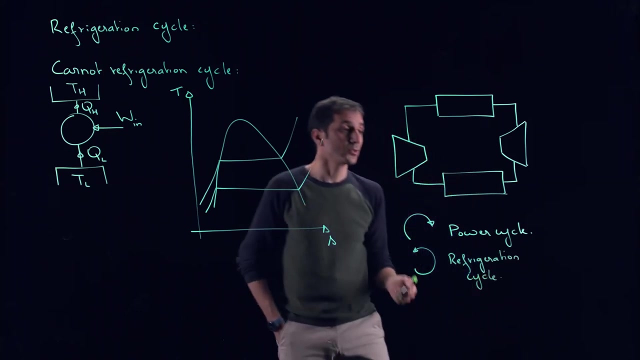 heat here. okay, so now, basically, if you run it this way, so clockwise, this is a power cycle. obviously this is only for a reversible cycle, and if you run it counterclockwise, you have a refrigeration cycle. So for us, we would like to run it anticlockwise. 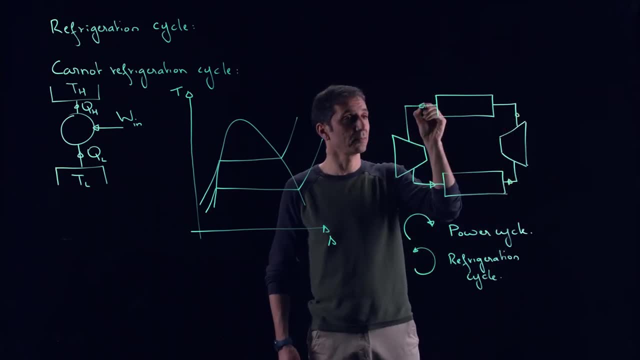 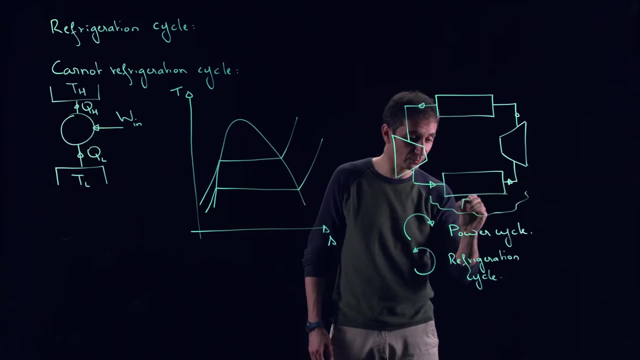 so, basically, we'll be going in this direction. So here, what do we have? Your food or the thing that you would like to cool down is sitting here and you would like to extract heat. So this is your QL here. 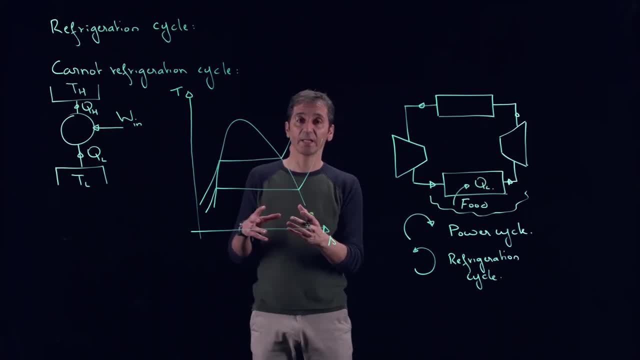 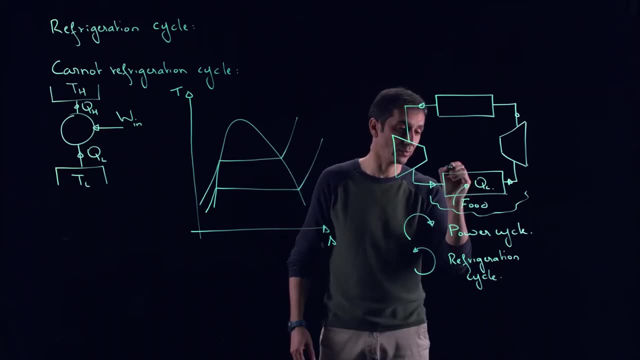 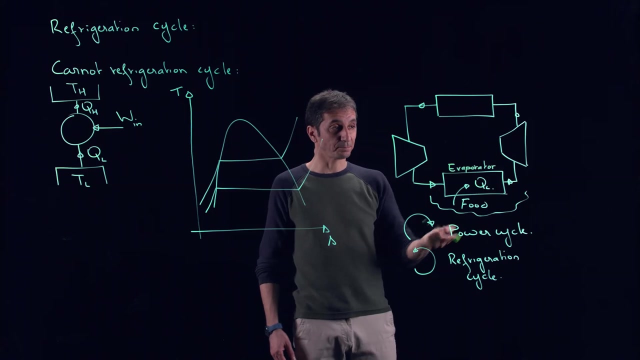 And to do this, what you are doing, you take a substance and then that will evaporate, that will have to steal heat from your food to evaporate, and we call this an evaporator. Okay, Then you will have actually to provide work here. 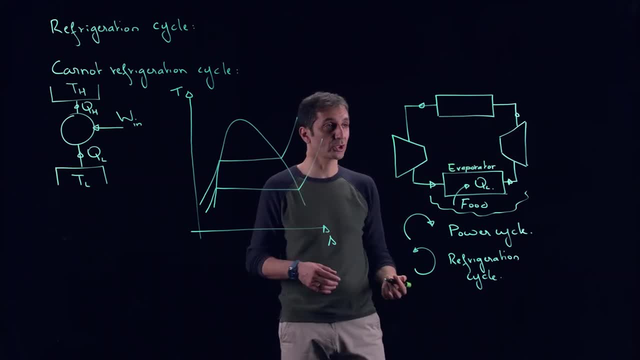 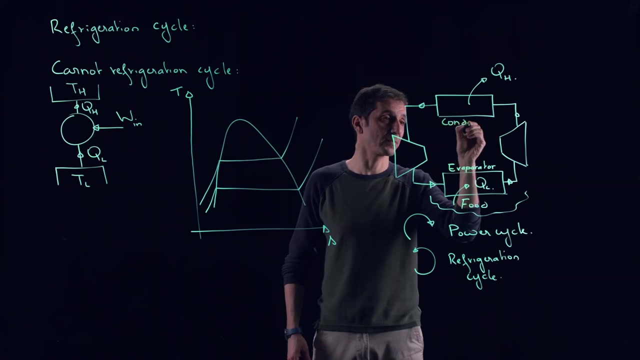 and then your refrigerant will go typically at the back of your fridge and reject heat to the surroundings. okay, So this will be your QH, And to reject heat, your actual refrigerant has to condense, so therefore we call this a condenser. 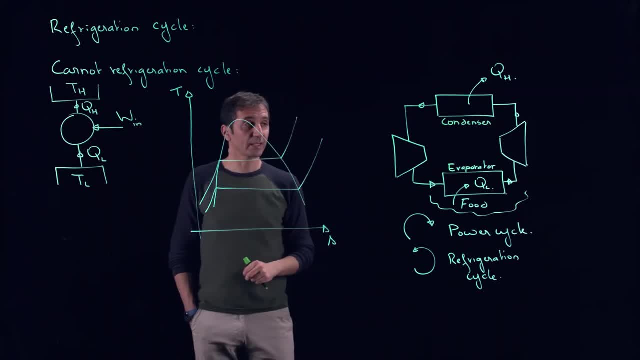 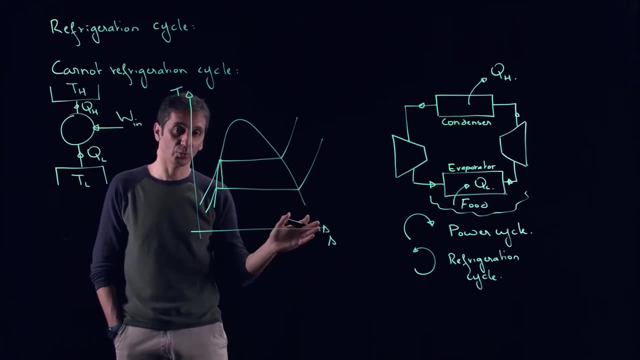 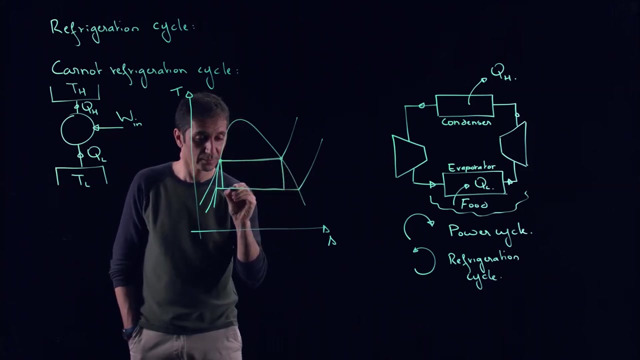 Okay, So now, basically, if we sketch our TS diagram here, what do we have? We will have the Carnot cycle. we have two isentropic, two isothermal. so it will be this. here are the different processes, and we are rotating. 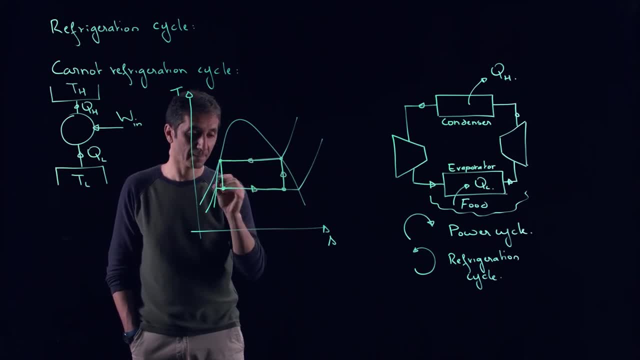 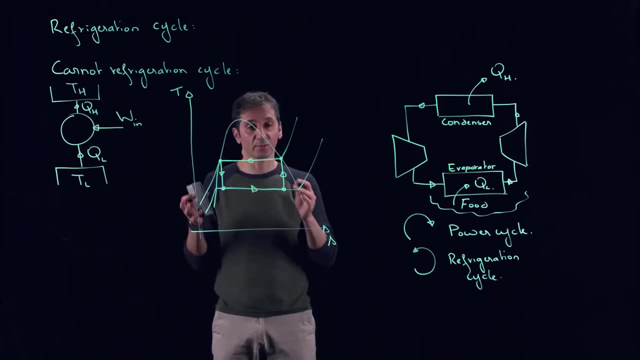 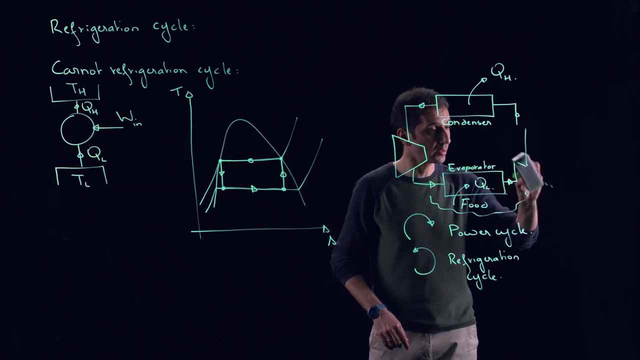 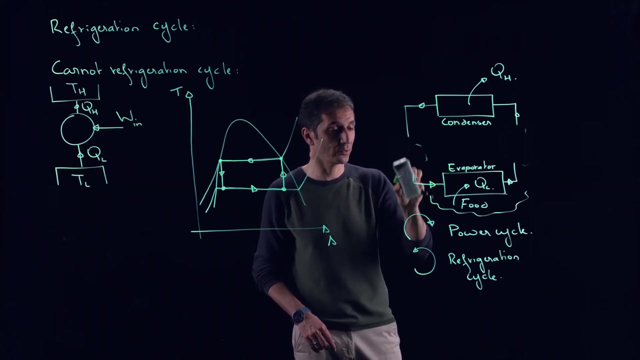 anti-clockwise. ok, so now, why, actually there is a problem with our kernel cycle. ok, we can identify different issues, and one of them is that now, basically, we are providing work here, so this one becomes our compressor and this one becomes our turbine- ok, we are running it in the other direction, right? so here now we have our 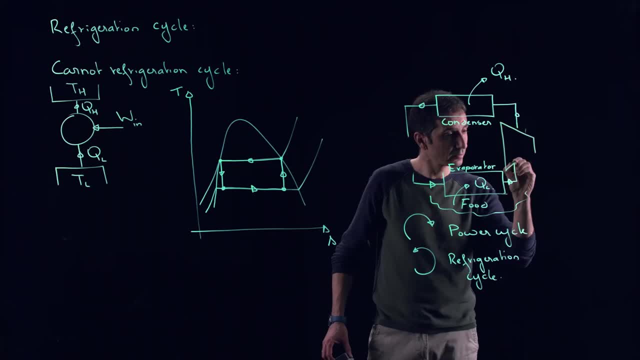 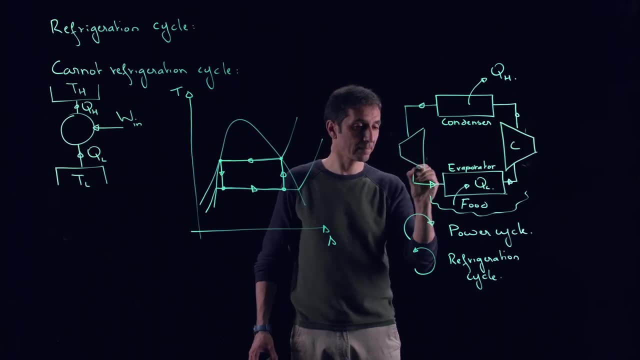 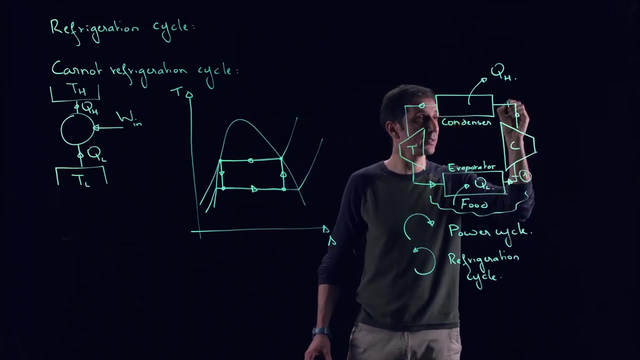 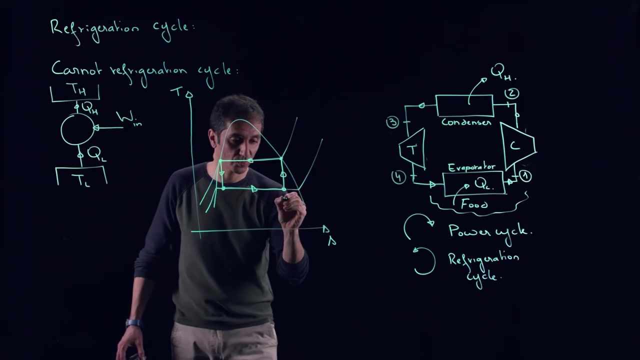 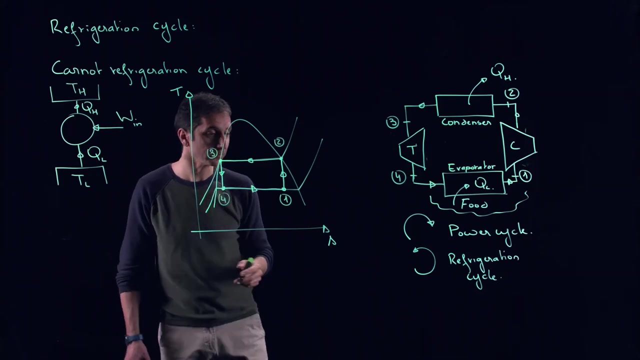 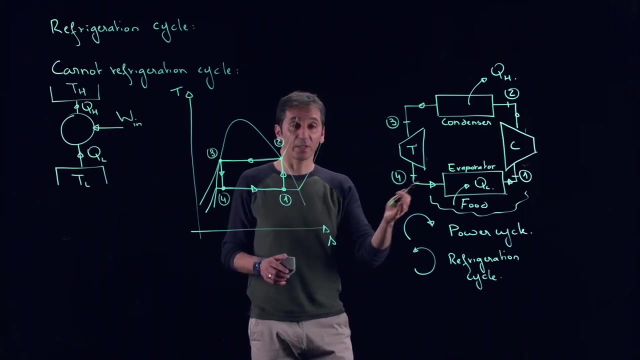 compressor and here we will have our turbine. first thing, ok, if let's say we put this state one, stage two, state 3 and state for, so this will be state 1, state 2, state 3 and state 4, the first thing we can see is that state want to stay to our compression. so 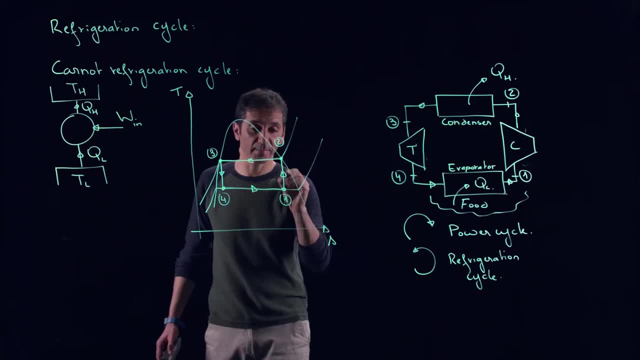 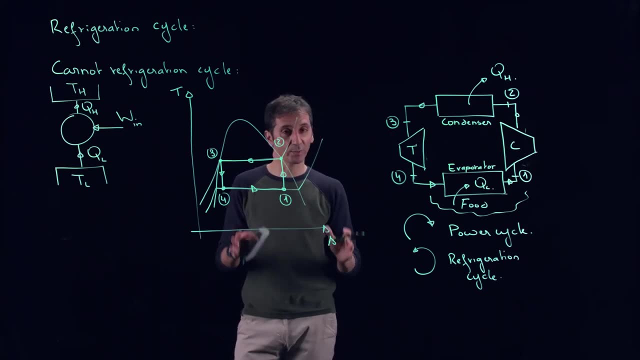 therefore, are using a compressor. however, you see that this is in a mixture phase. okay, and this is something we don't like. okay, we don't like, basically, when we have a mixture and we try compressor, we really prefer to have liquid. so you use a pump or a vapor a. 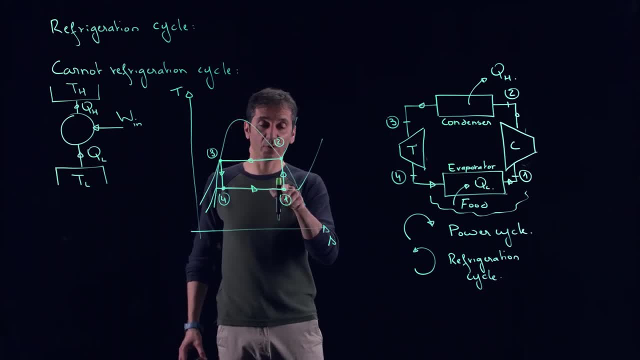 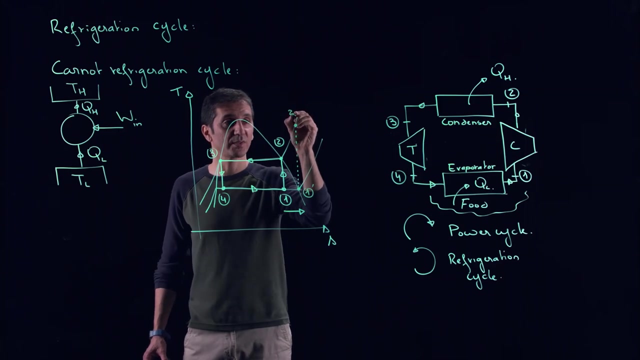 gas and you use a compressor. so basically, it's really problematic for us to have this point one in the mixture phase. the solution is that we will move it to the right, so our new state one will be here and since the process remains isentropic, this will lead us to this new state to prime. so our fix in 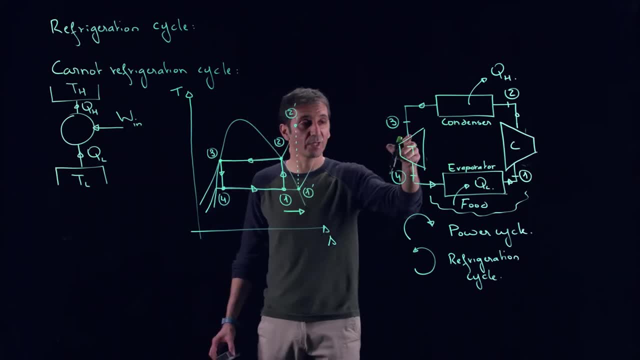 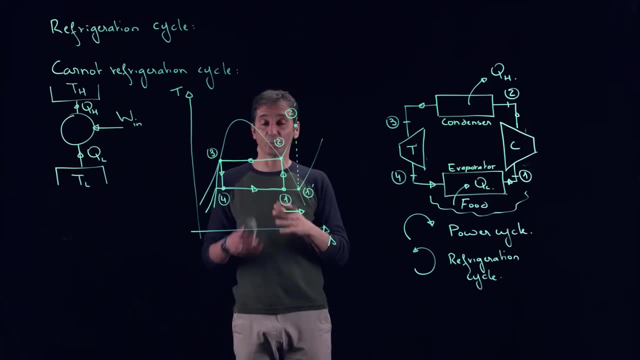 this then the other thing is that you see, here we have the turbine, and this is complicated. why? because the only lower role of the turbine is to create an expansion process and to reduce the pressure from 3 to 4. okay, that's it, ideally, with the turbine, it would like to. 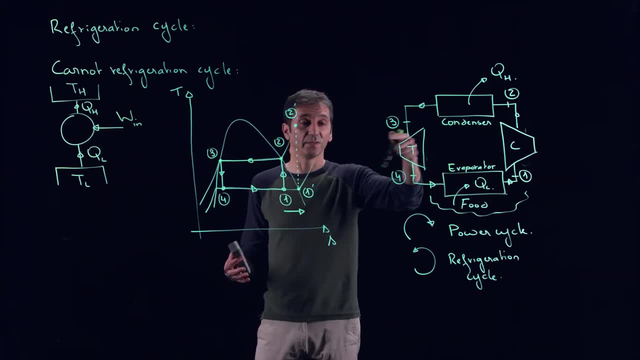 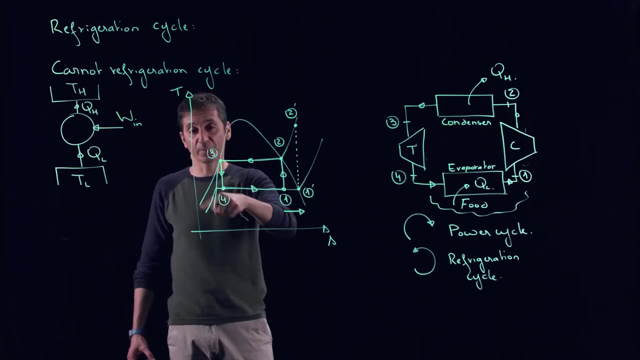 just reduce the pressure and get rid of the pressure so we can get rid of the generate power. But here, basically, the difference in pressure: you are not in the superheated region, right? You are close to the compressed liquid region or with qualities. 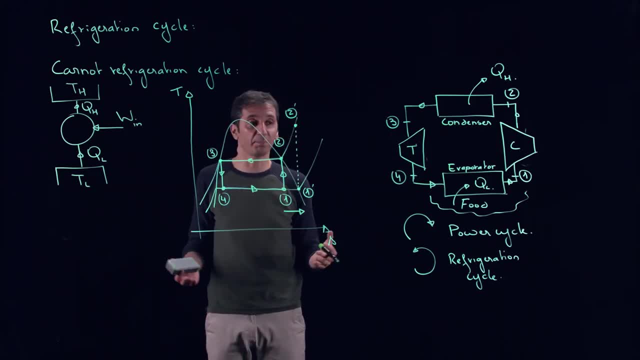 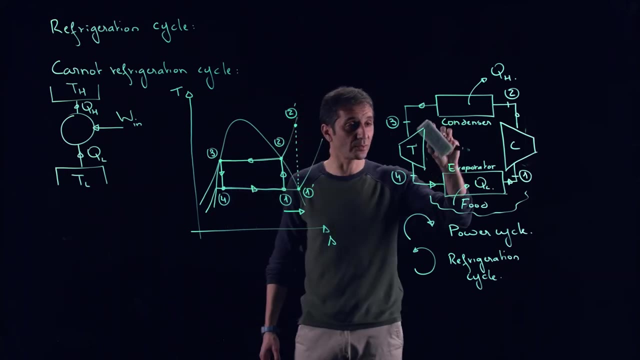 very low qualities. So, basically, you get simply peanuts out of this turbine. So you are making your life very complex, using complex equipment in order just to reduce your pressure. So the solution in this case is not to use a turbine. We will simplify this.